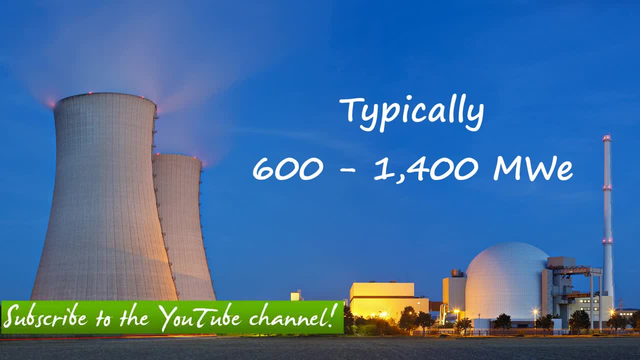 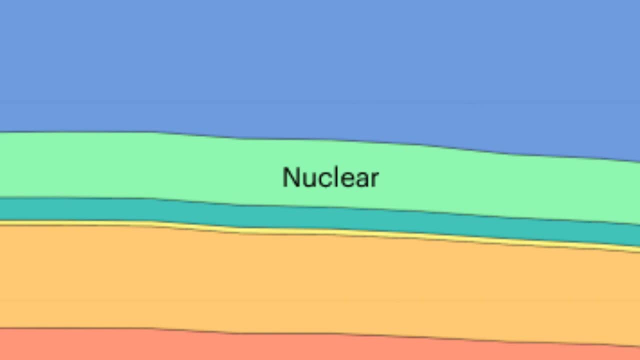 If we were looking at the entire nuclear industry and how much of the world's power is produced by nuclear energy, then nuclear power meets currently about 5% of all our requirements. But it depends a lot upon your geographical location, For example, in France. 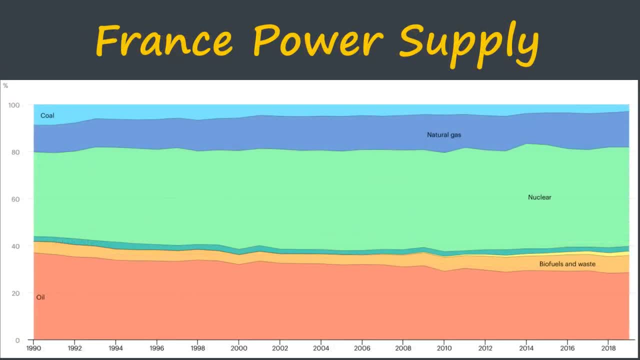 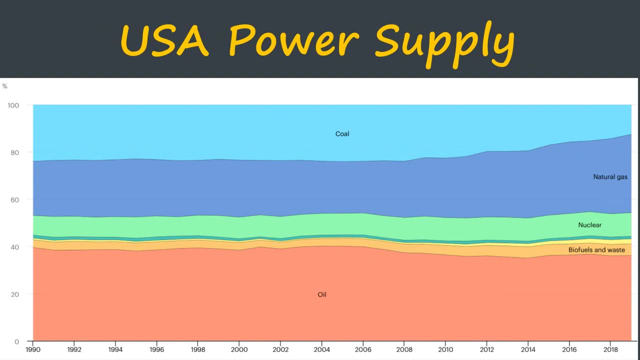 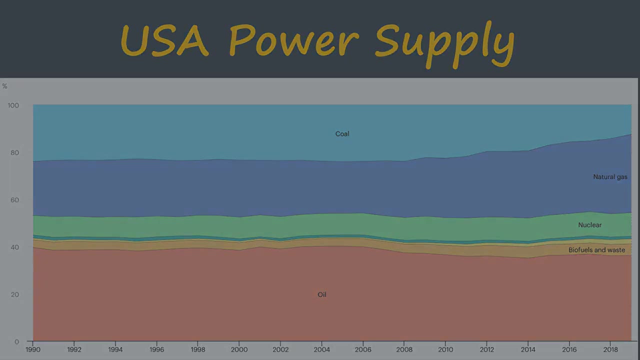 they rely heavily upon nuclear power In the USA, although they have a larger installed nuclear megawatt capacity than France, they rely on it far less because they get energy from other sources, for example coal, gas and hydro. So before we have a look at a boiling water reactor? 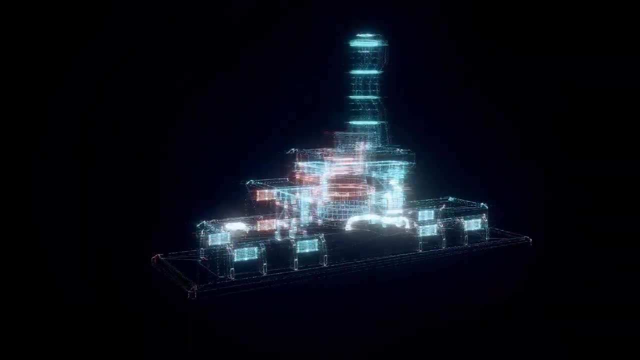 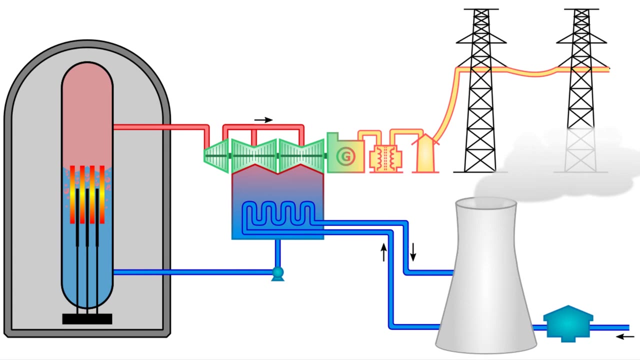 and the components, let's have a look at how it works and why we need a boiling water reactor in the first place. So here's a nice simple diagram showing exactly how a boiling water reactor nuclear power station works. Within this gray building, the containment building. 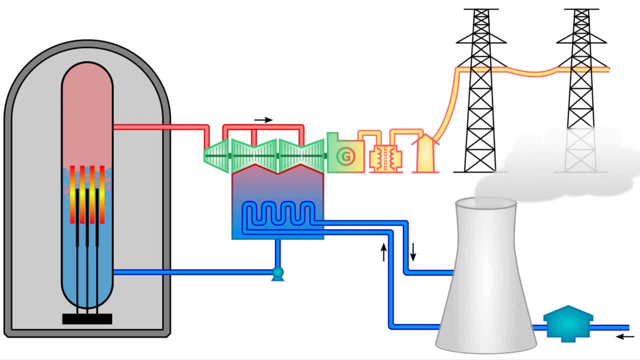 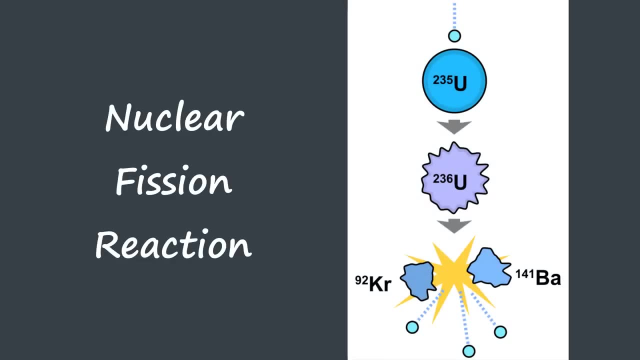 we have our boiling water reactor. It is essentially our heat source and we're gonna take that heat and use a lot of other machinery in order to generate electricity. So the big question here is how can we take a nuclear fission reaction, that is to say, splitting of atoms? 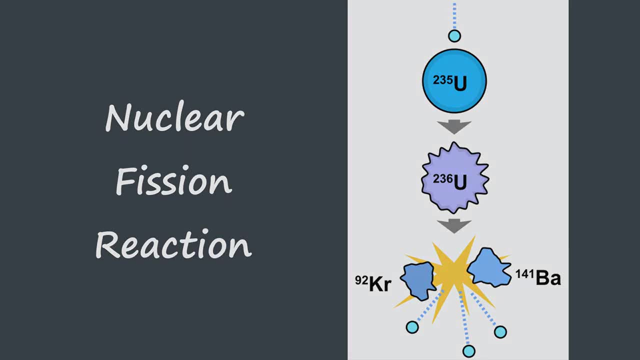 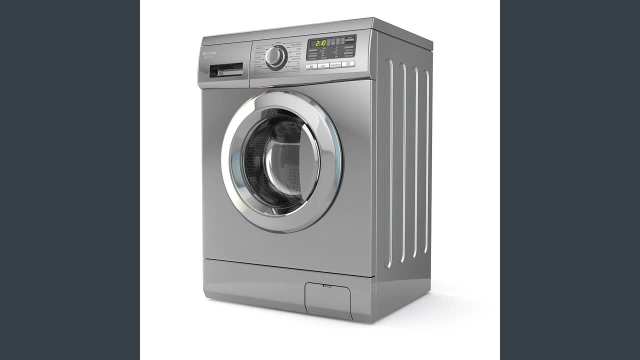 and turn that into electricity that we can use in our homes to boil the kettle or make the washing machine run, or so we can watch TV, et cetera. Well, let's keep the scientific stuff really basic. The nuclear reaction that's occurring: 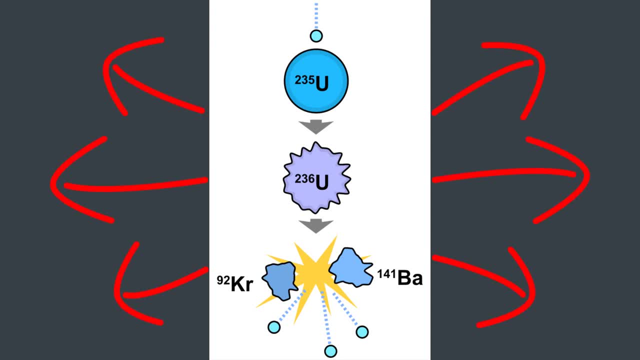 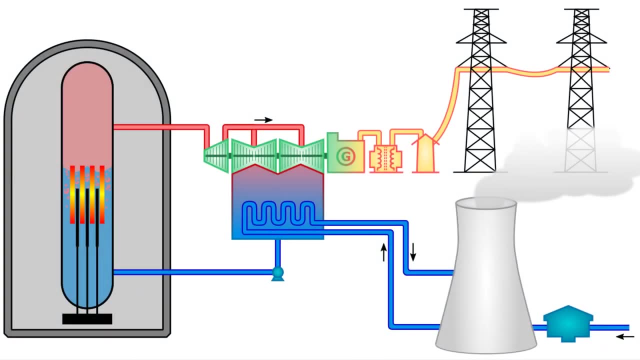 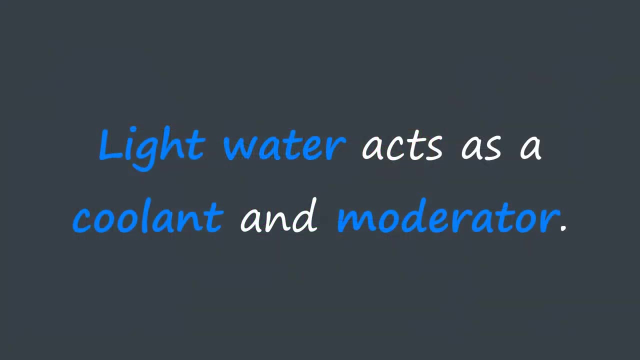 in our boiling water reactor is creating heat. That's all we need to know. How are we gonna turn this heat into electricity? We submerge our boiling water reactor in water, specifically light water. This demineralized water acts as both a coolant and a moderator. 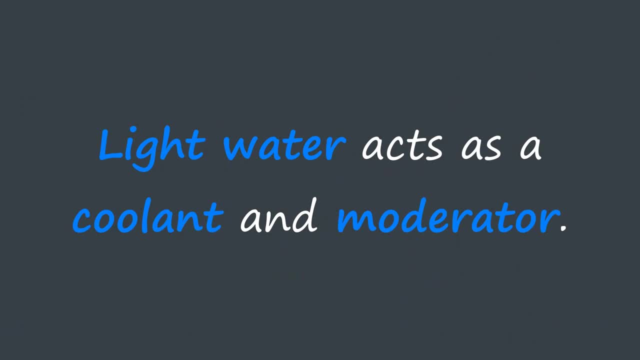 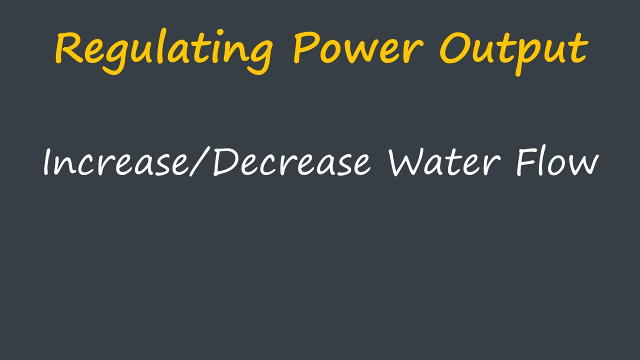 Coolant means it keeps the reactor cool, and a moderator is just something we can use to control the rate of reaction within our reactor. We can increase or decrease the power out from the reactor by regulating just how much water flows through our reactor- Another way to regulate the power output. 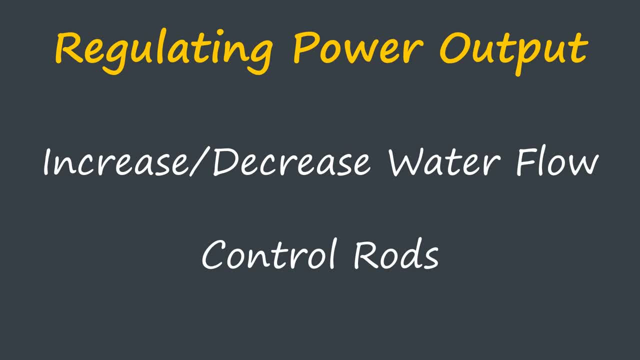 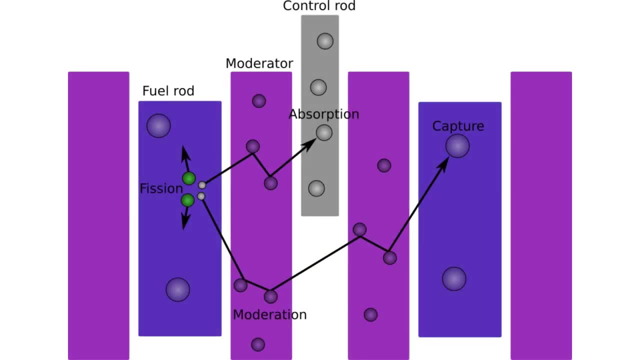 is by using control rods. Control rods are slid into and out of the reactor in order to absorb neutrons and slow down the reaction or not. We'll look at all of these parts in a moment, when we go through the boiling water reactor in more detail. 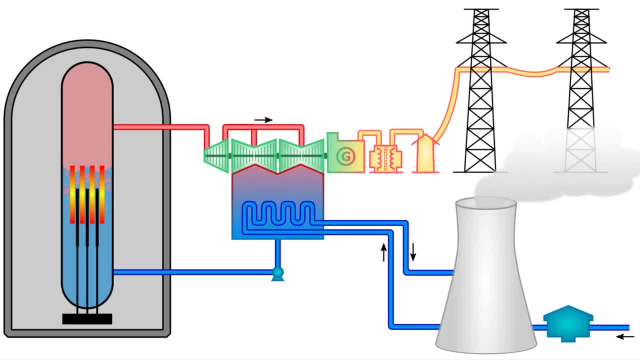 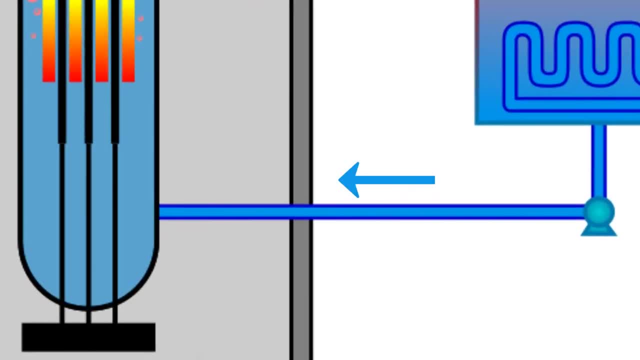 So we've got our heat source. We can regulate how much heat we're generating using control rods or our moderator, which is demineralized water. Feed water is fed into the reactor and is heated up by the reactor until a percentage of it turns to steam. 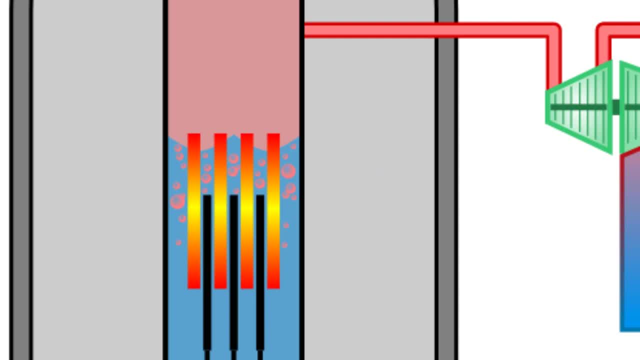 typically about 15% of it, based upon mass. The produced steam then leaves the reactor and is passed to a steam tank. That's what we're gonna do. That's what we're gonna do. That's what we're gonna do with the steam turbine. 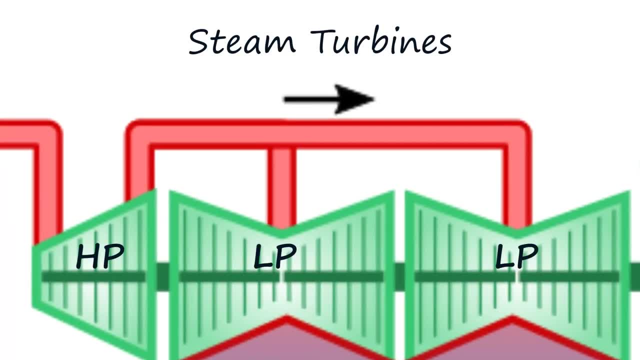 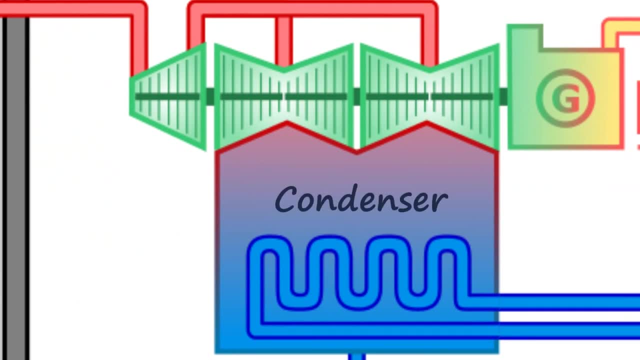 We pass the steam to a high-pressure steam turbine, then a low-pressure steam turbine and then, finally, we'll discharge the steam as exhaust steam to a condenser, and the condenser cools the steam so that it changes state and becomes a liquid. 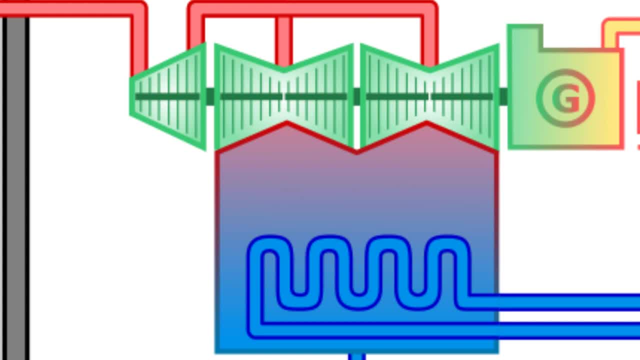 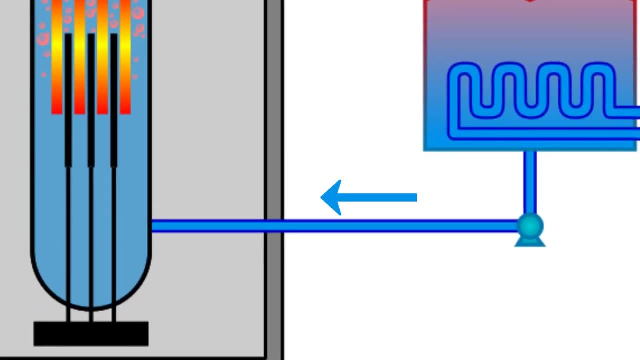 The water that accumulates at the bottom of the condenser is not called water, It's called condensate, And once it's been reheated and treated, it's pumped back to the boiling water reactor and we classify it then as feed water. 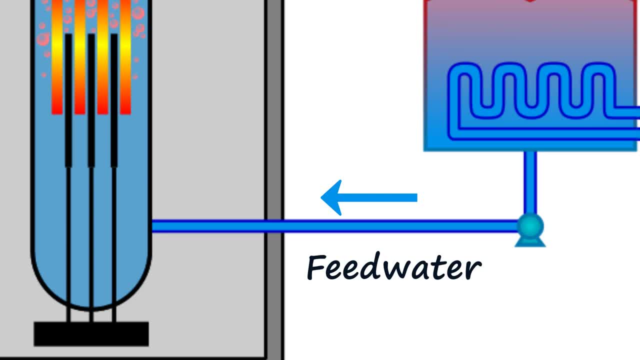 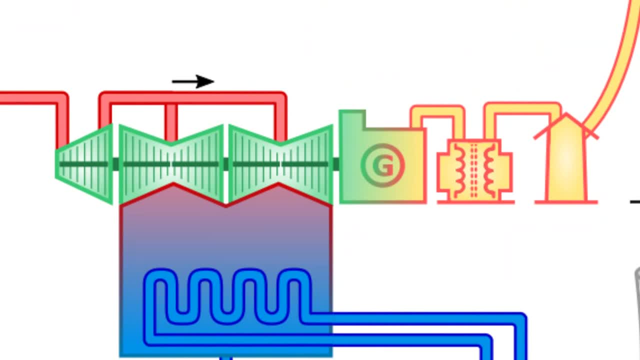 because it's being fed to our boiling water reactor. When steam passes through the steam turbines, it causes the turbine rotor to rotate and we connect our steam turbine to a generator. The rotor within the generator rotates and we begin to generate electrical power. 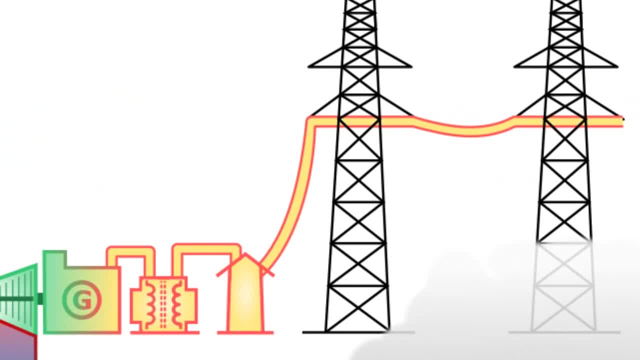 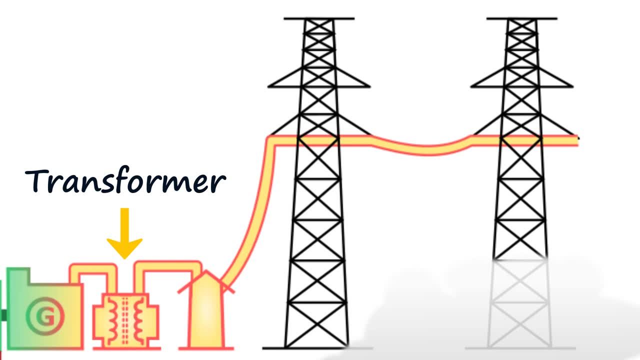 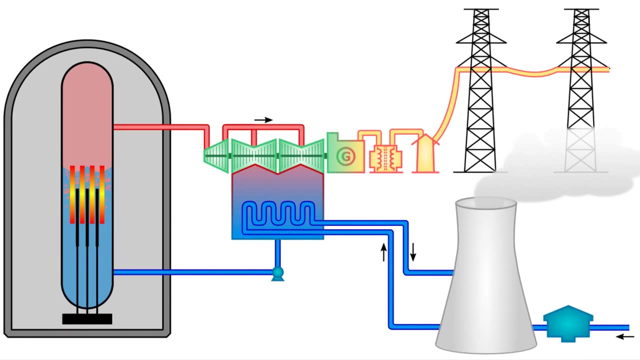 We then distribute this power via a electrical transformer, a substation, and then into our electrical grid. Although we talk about generating power, we're not actually doing it. We're not generating anything. It's not possible to generate energy. We're only ever transferring energy. 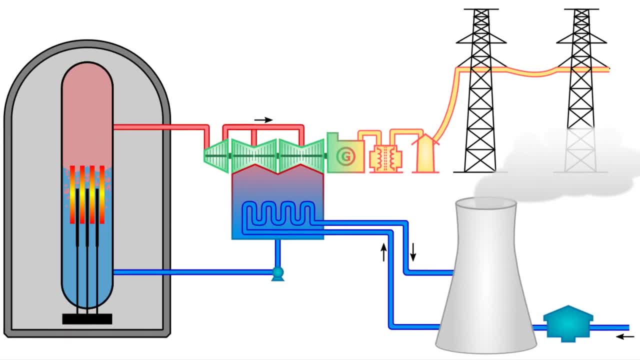 from one place to another. In our example here we're taking the heat energy from our nuclear reaction, transferring it to our demineralized water, then to steam, Then we transfer the heat energy to the turbine so that we have mechanical energy. 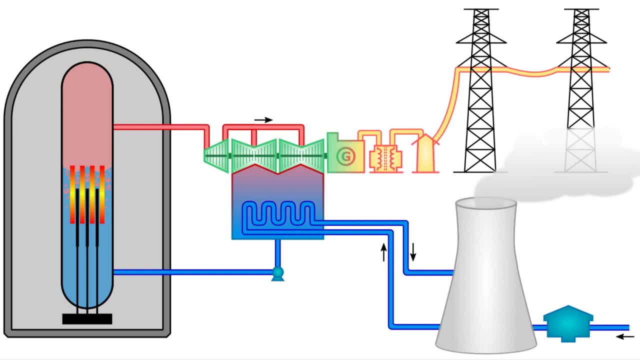 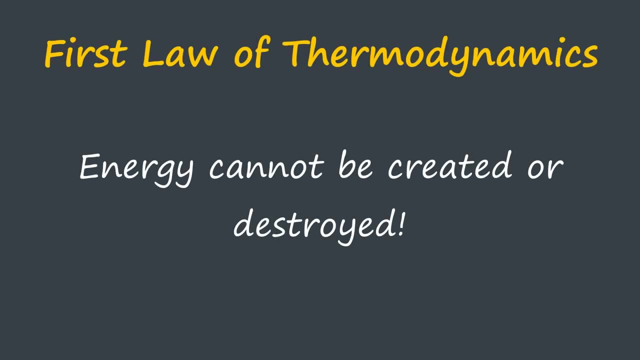 because the turbine begins to rotate And finally we change that mechanical energy to electrical energy and we have a generator. So the entire process is simply a energy conversion process. If we could find an easier way to generate electricity without having a nuclear reactor and turbines, et cetera. 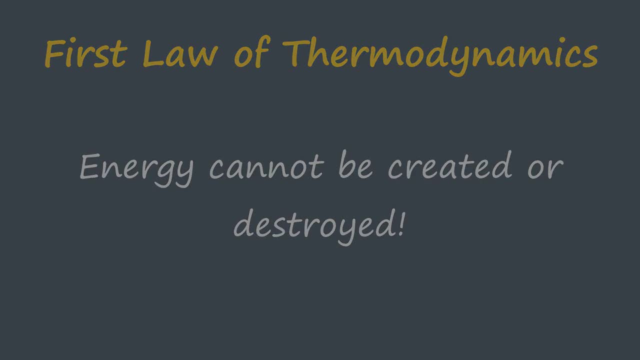 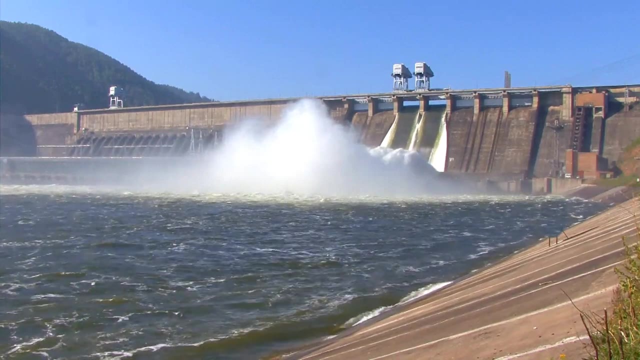 then we would already do this. If you ever look at hydro power plants, they don't require a heat source, which means they require far less equipment and machinery than a nuclear power station does, or a coal-fired power station, et cetera. 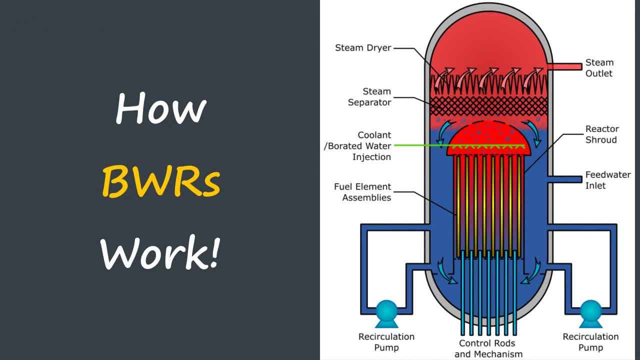 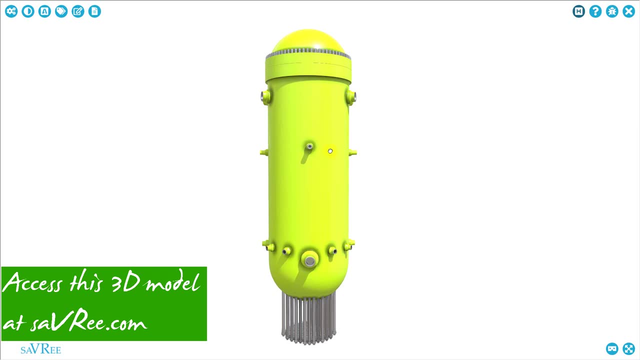 Now we know what the boiling water reactor is doing and why we require it to generate electricity. Let's go and have a look at some of the parts and components that make the boiling water reactor work. Here is a boiling water reactor. Let's do a little spin. 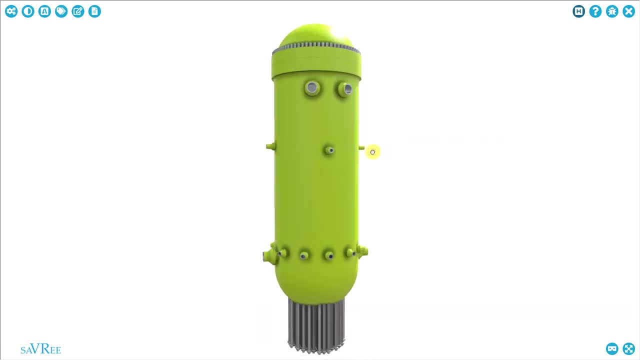 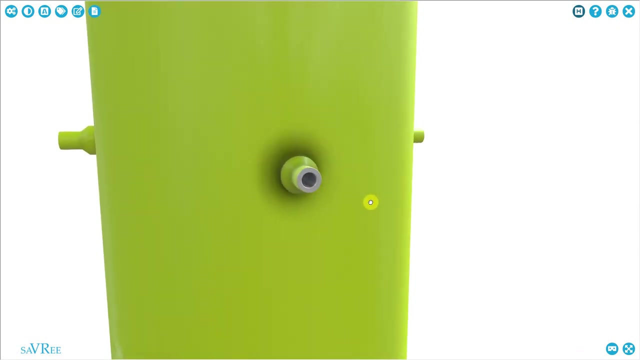 It's long and cylindrical in shape and it would sit normally within what's called the dry well within the containment building. You can see there are a lot of penetrations that go through the BWR. some are quite large. This one here as an example is quite small. 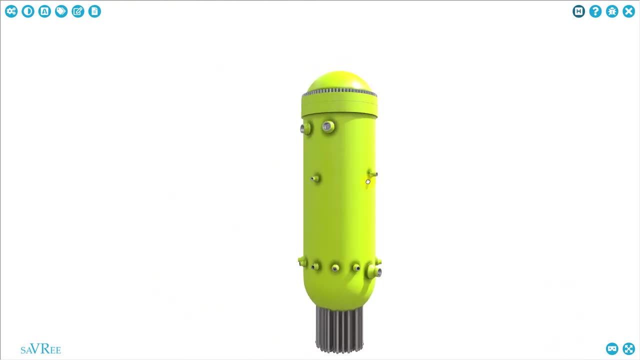 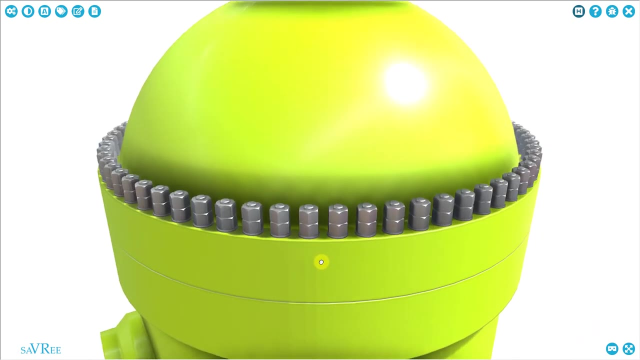 The green item that we're looking at is called the vessel. The item on the top is called the vessel head, and the vessel head connects onto the vessel body or the vessel via studs and two nuts. We tighten up the nuts hydraulically. 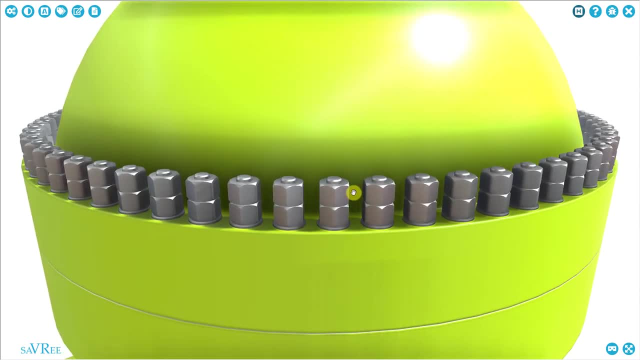 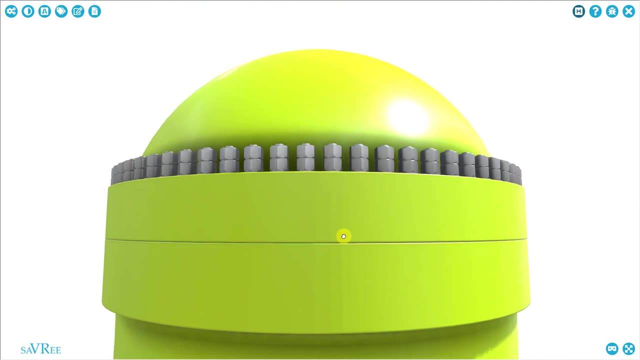 The top nut is a locking nut and that's there to ensure that the lower nut does not come loose over time. We've got a couple of O-rings to seal the space between the vessel head and the vessel and these two O-rings. 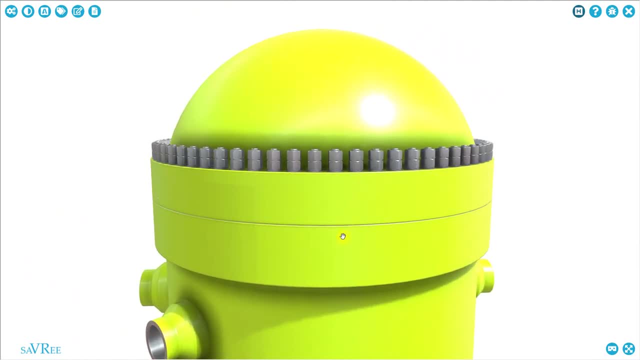 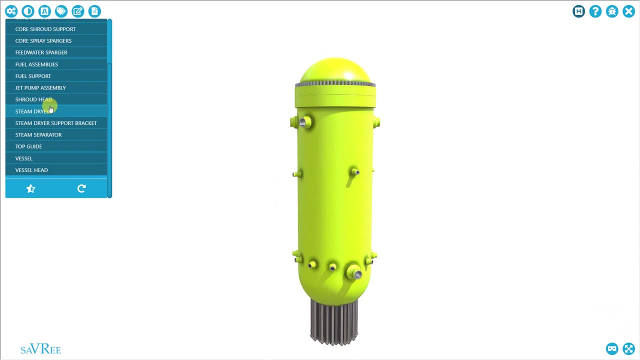 they're actually quite thick. pieces of metal are crushed between the vessel head and the vessel. That's what allows us to create a seal. If we use our configurator, we can actually take a look at the parts- vessel, vessel, head- and then we invert. 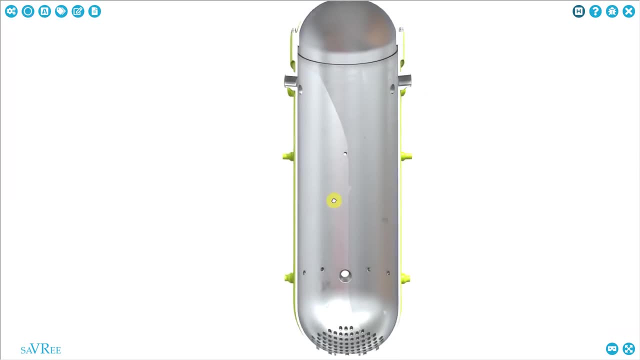 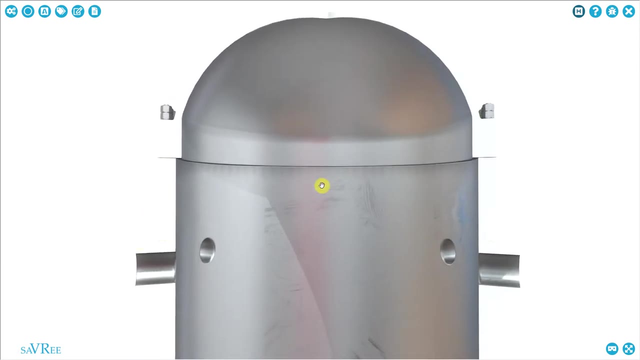 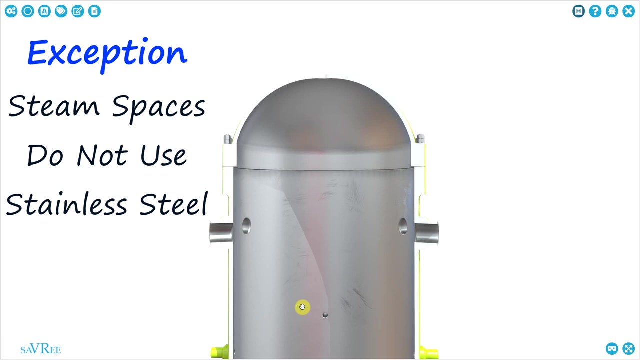 and if we take a cross section, you can see how it looks on the inside. The inside of the vessel is coated or clad in stainless steel. The bits that can't be clad in stainless steel are manufactured from a nickel-chromium-iron-based alloy. 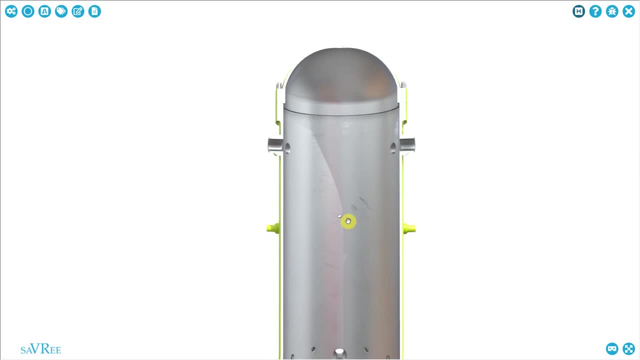 which has similar properties to stainless steel, and thus everything within the vessel is very corrosive resistant. If we look at the penetrations, we've got steam that flows out of these penetrations at the top. Come further down, we've got feeders. 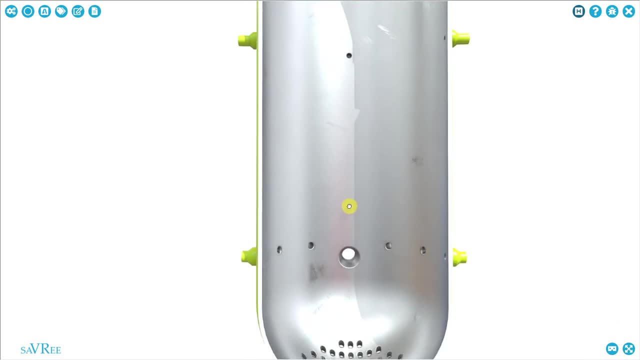 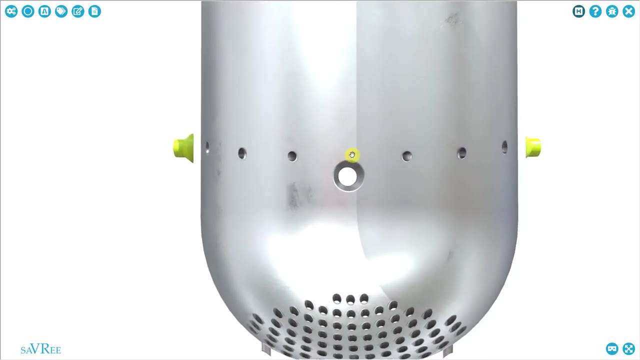 we've got feed water inlets as well as the emergency cooling inlets Further down still. we've got some connections here and these feed to jet pumps. We'll talk about those in a moment. The jet pumps are the smaller holes. 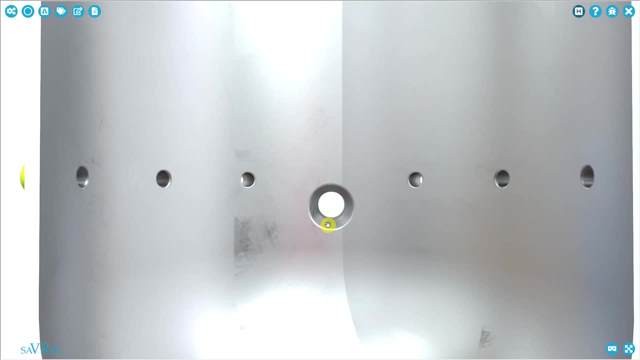 and the recirculation pumps. the suction is through this bigger hole in the center of the screen, So floated jet pumps coming in through the small holes here, suction to the recirculation pumps, out through the big hole here, and what you have to realize is that when we 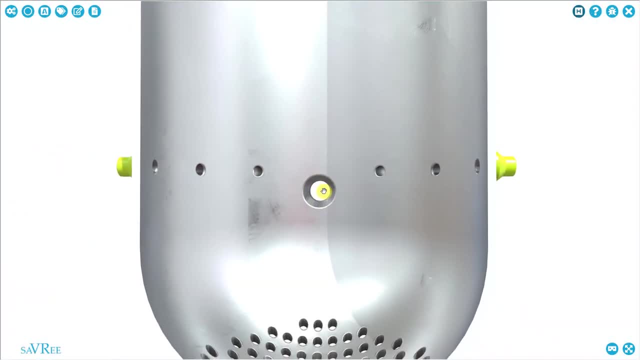 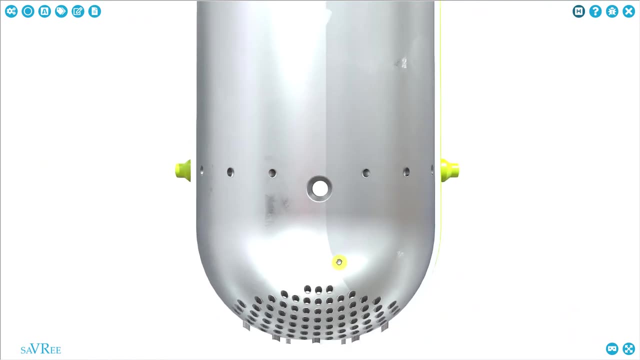 suck demineralized water out through the large hole in the middle. it's coming back into the vessel through the smaller holes, So it's a closed system. apart from the fact that some of that water will turn to steam as it passes through the reactor. 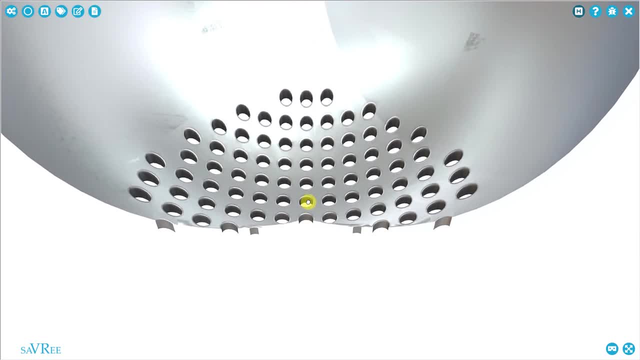 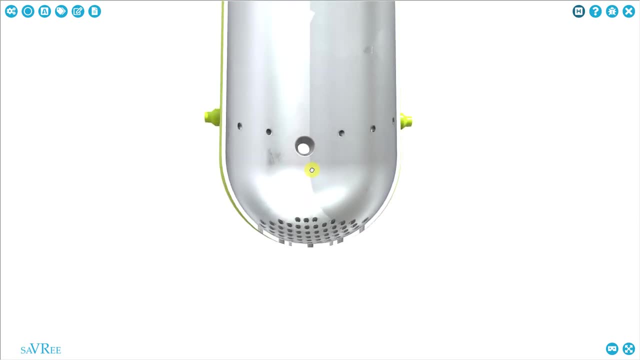 At the bottom of the vessel we have these penetrations that allow our control rods to pass into and out of the vessel. As mentioned previously, we use the control rods to slow down the reaction and thus to regulate our reactor power output. Let's put the parts inside our little reactor. 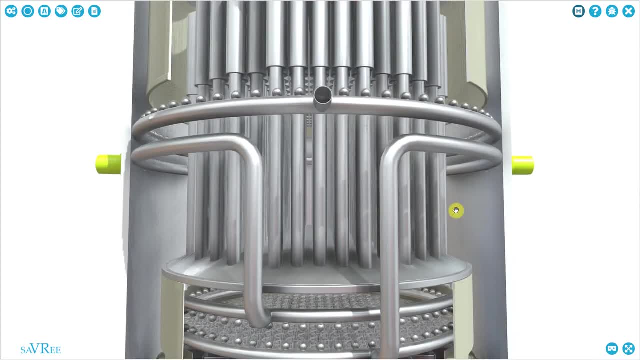 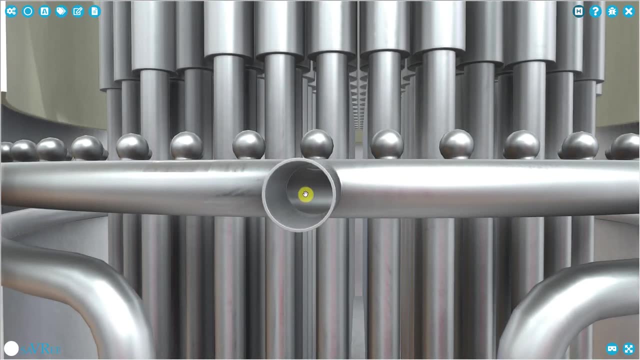 and we'll work from the feed water inlet downwards. We've got our feed water inlet, This is our feed water, sparge pipe. Feed water comes in through this connection. It flows into this sparge pipe, this circular ring with these nozzles on it. 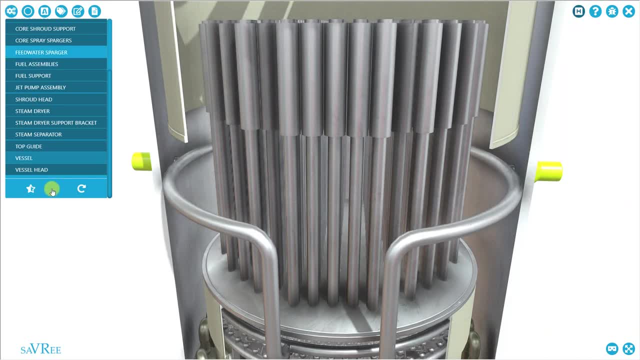 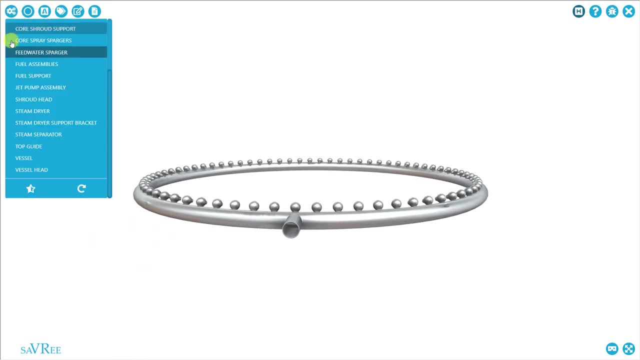 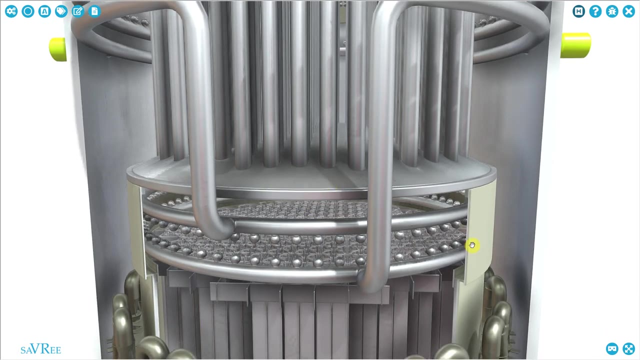 In fact, if we configure it, we can take a better look. There you go: We're spraying feed water into the middle of our BWR. The feed water then falls due to gravity and it's going to drip down. It's the top cover of our shroud. 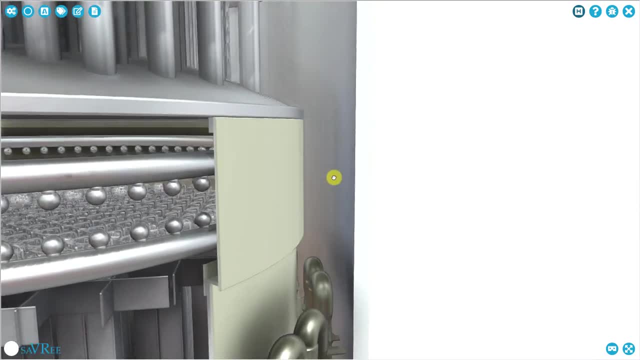 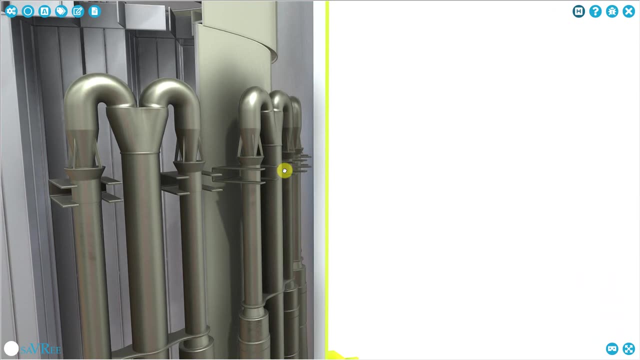 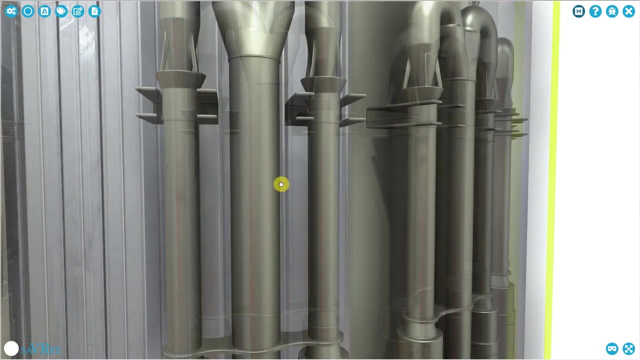 and flows down between the shroud and the vessel. This space is called our downcomer area. As the water flows down, it actually gets taken into this item here, which is a jet pump. You can see from this angle that the water would come up here. 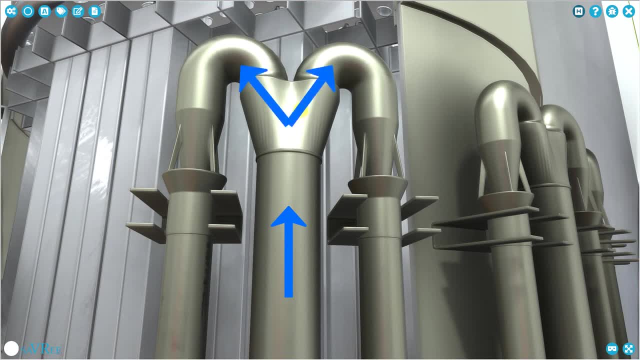 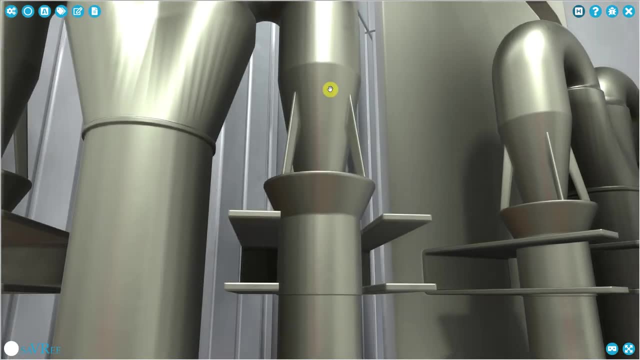 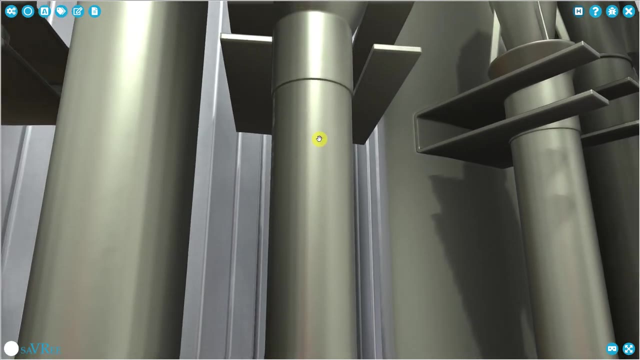 This is our jet pump riser and then it splits off in two different directions and then its velocity increases as it passes through this nozzle and it flows into a mixing tube. That is this lower mixing pipe or mixing tube here, As it flows down through the nozzle. 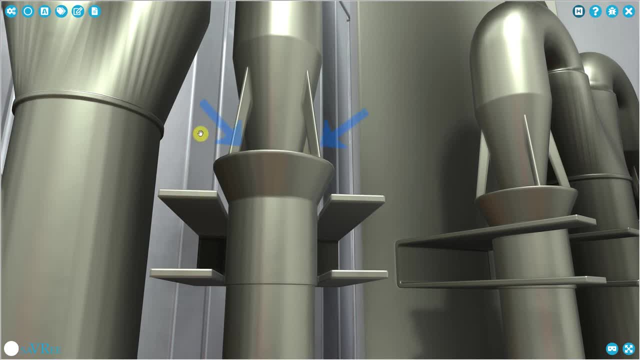 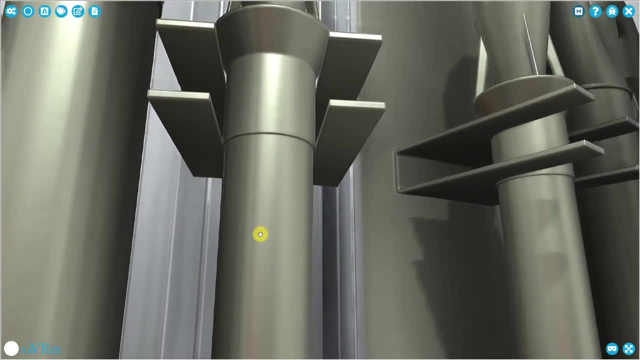 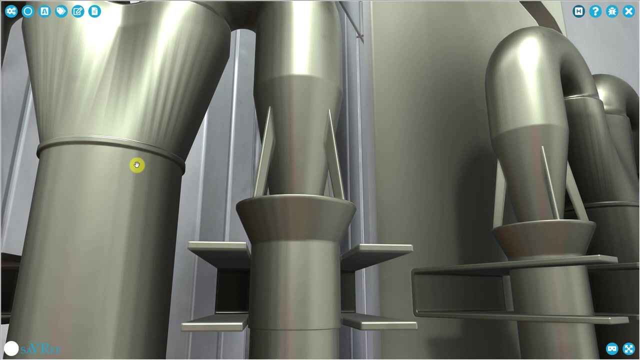 the nozzle is open and water is drawn in from the sides into this funnel where my mouse is, and then we get mixing of the feed water- that is, the relatively low pressure water that's being drawn into this funnel- and the recirculation water. 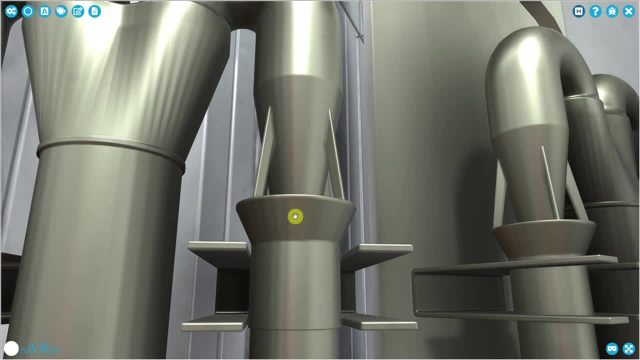 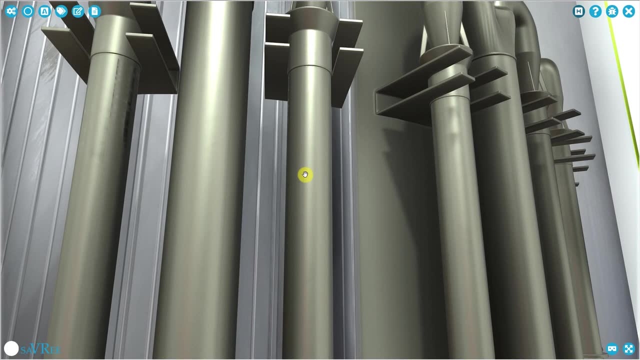 which is the water that's coming out of this nozzle, So we'll mix those two together. About a third of what passes into the mixing tube is recirculation water, with the remainder being feed water. The water that's mixed comes down here. 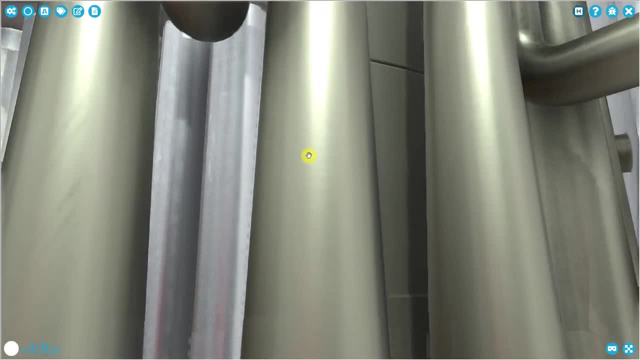 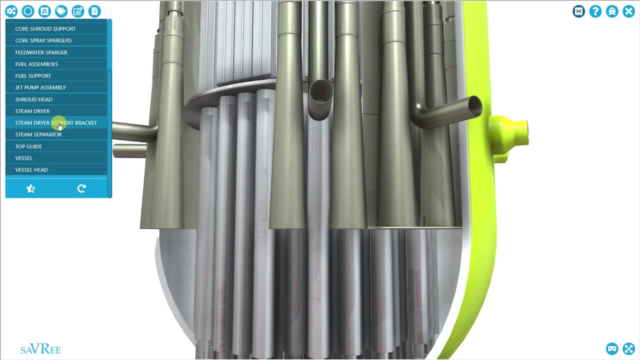 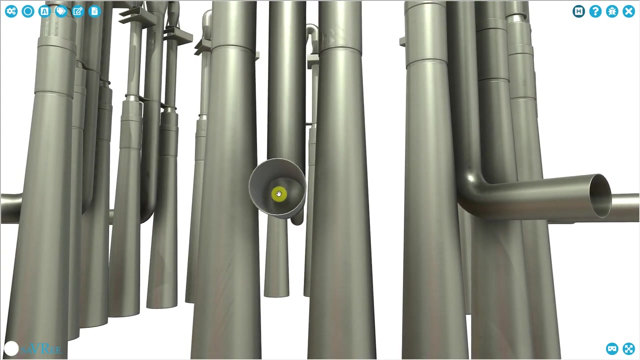 and passes out of a diffuser. See if I can find our jet pump diffuser. You can see it there. In fact, if we use our configurator again, we can have a better look. There we go, So you can see that the water would enter through this pipe. 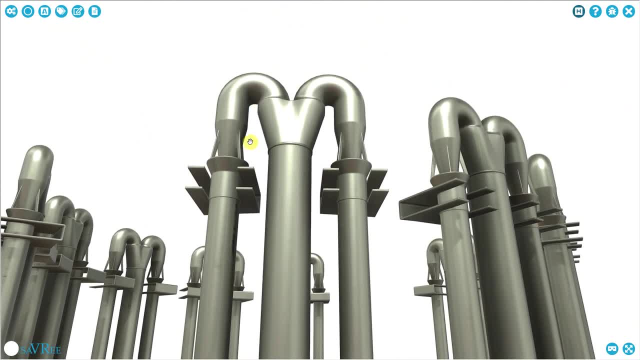 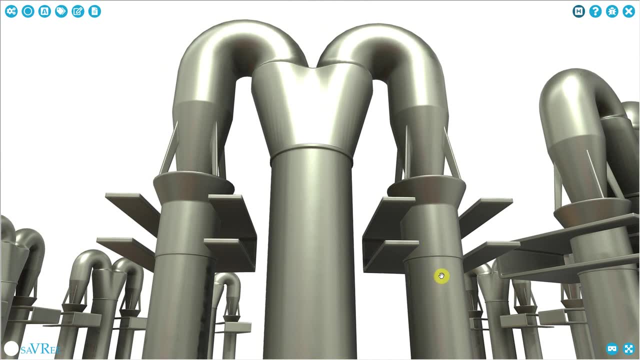 comes up through the riser, splits off. that's our recirculation water that splits off, comes down through the nozzles and is sprayed at high velocity into the mixing tube or the mixing pipe and from the sides. then 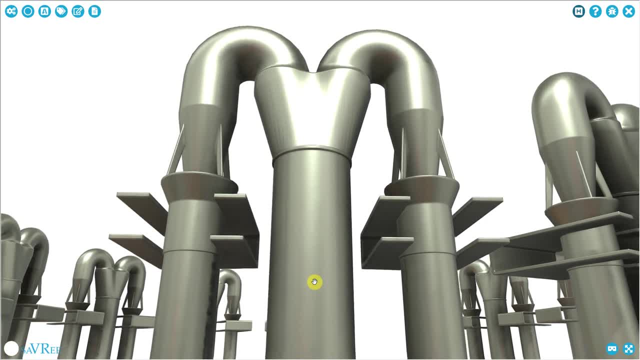 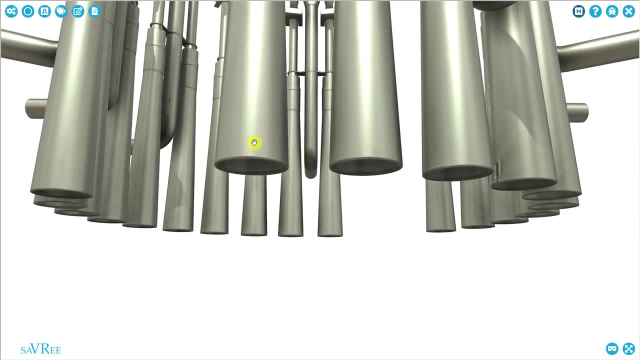 we draw in our feed water. When the feed water and the recirculation water is mixed, then we will discharge that mixed water out of our diffusers, and there's two of these per jet pump. You can see the shape of the jet pumps here. 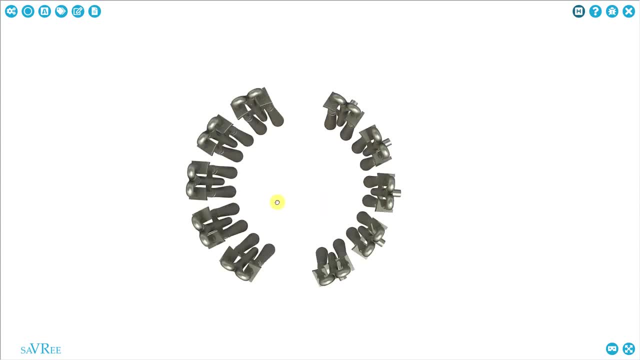 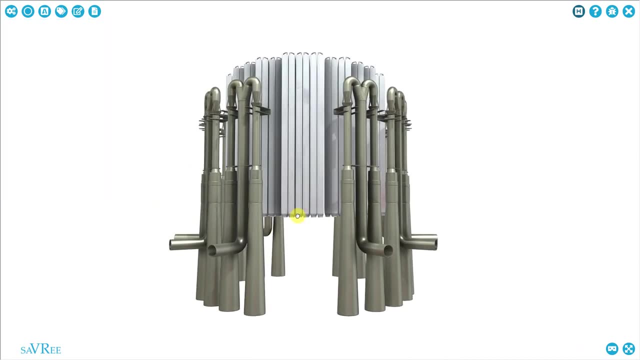 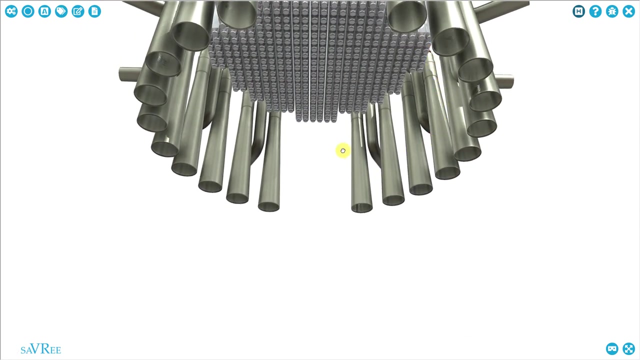 they're evenly spaced around our main reactor core. You can see the fuel assembly here and, based upon this perspective, what you have to realize is that the water's coming out through the diffusers at the bottom and is then going to turn around 180 degrees. 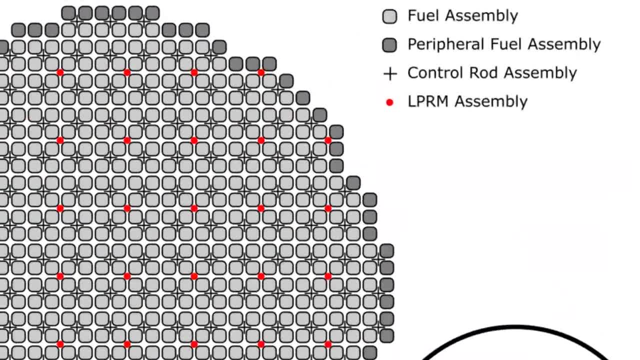 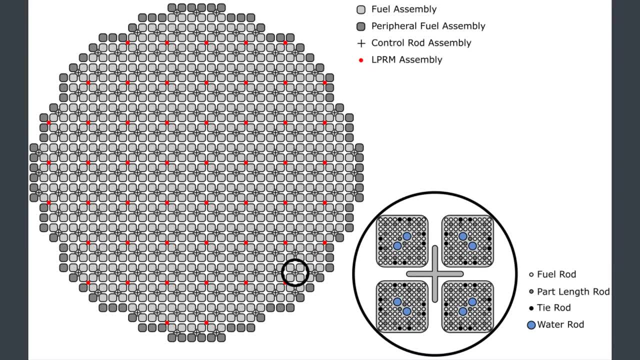 and flow upwards through our fuel assemblies. There'll be hundreds of these fuel assemblies and as the water flows it's going to become heated. Let's go back to our cross-sectional view and we can have a look at that in a bit more detail. 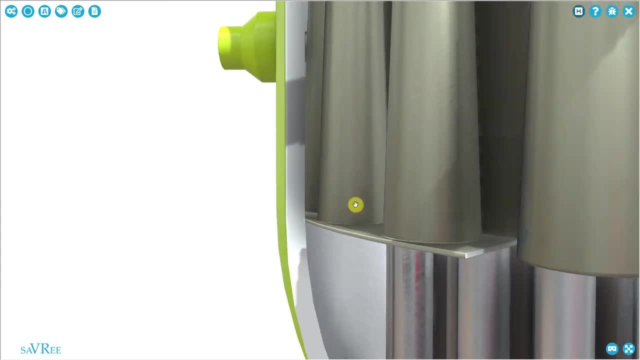 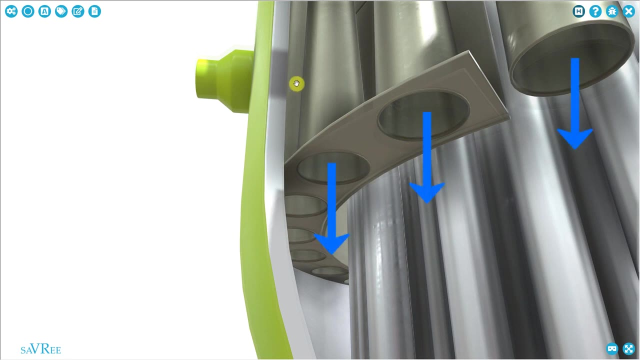 The water is coming out at the base of our diffusers. We've actually got this cover plate here that connects to the shroud and that's what stops the water from flowing: simply downwards. It has to flow through the jet pump, the feed water and the recirculation water. 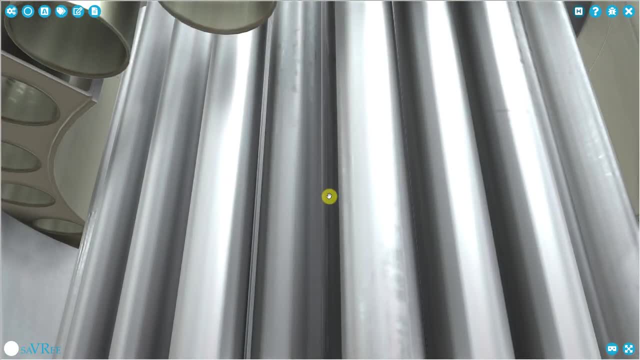 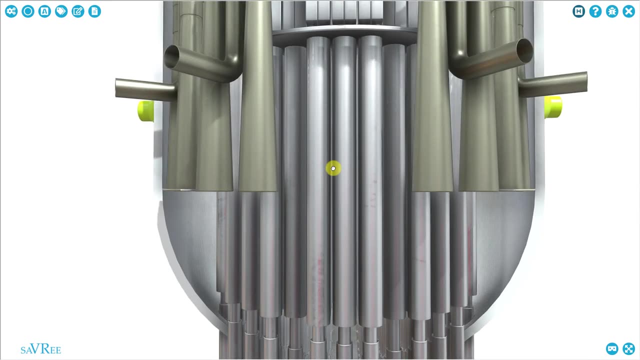 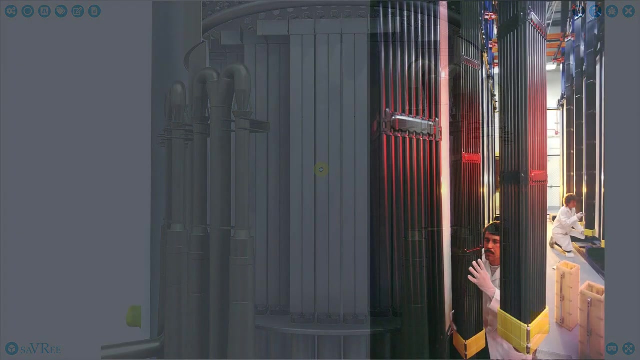 Comes out here and then it will flow around these other items for the control rods. These are the guide tubes for the control rods and the water will flow upwards through our fuel assemblies. A fuel assembly is represented by long, thin fuel rods. 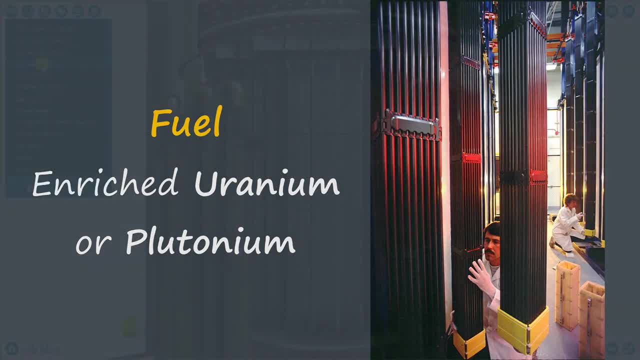 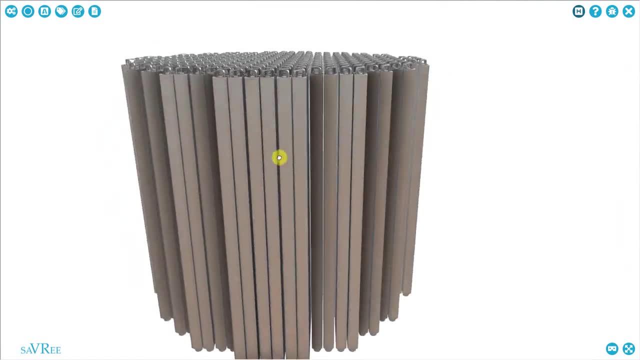 And it's within this space, where the fuel assemblies are, that our water will be heated. You can see them here. these are our fuel assemblies. We've actually got handles on the top because we remove head in order to get to the fuel assemblies. 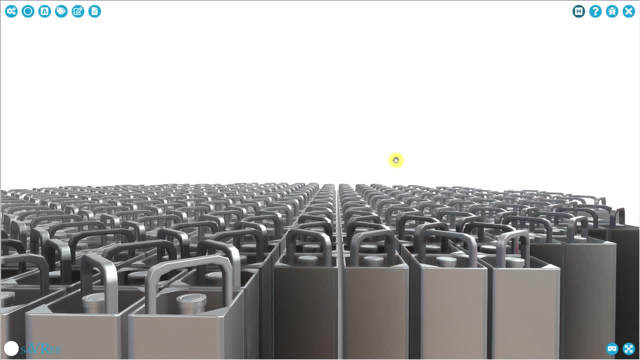 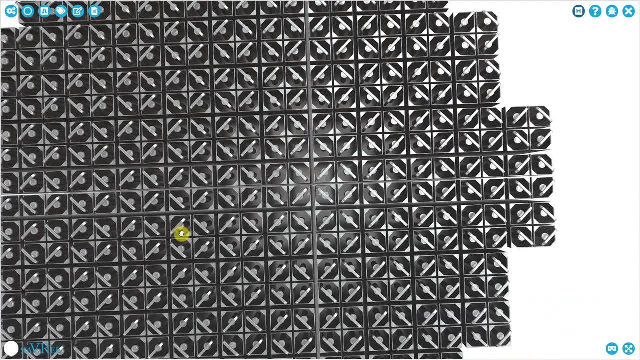 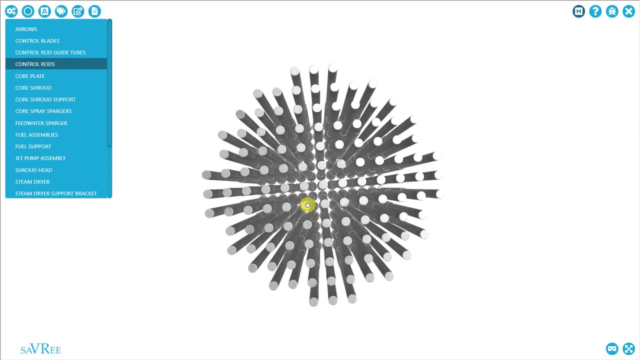 to pull them out and change them, maybe every 18 to 24 months, depending upon design. Between each of the fuel assemblies we will have control rods scattered around the top. You can see they're here. They're laid out in a pattern between the fuel assemblies. 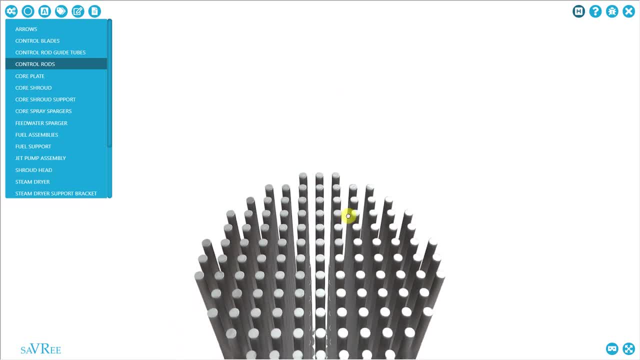 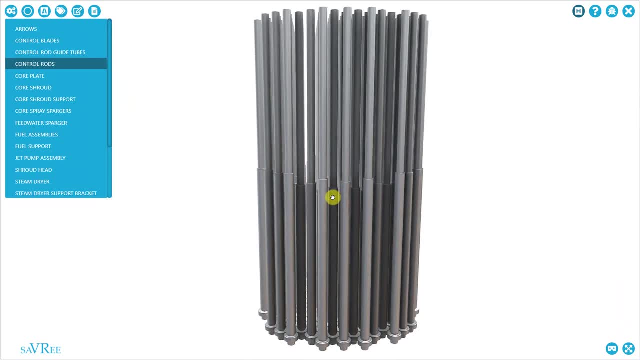 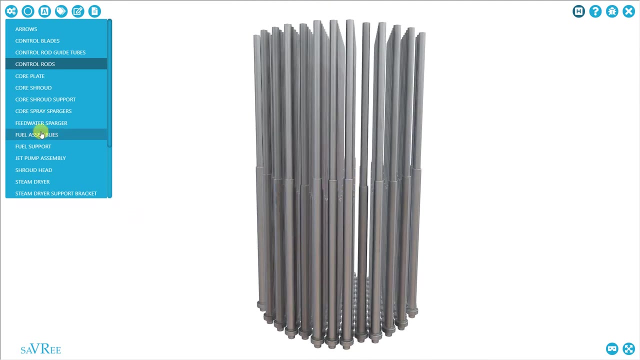 so that when we insert those control rods, we can slow down the rate of reaction and thus reduce our megawatt power output. or maybe we want to install the control rods for safety reasons, For example to stop a runaway reaction. What's unusual about the control rods? 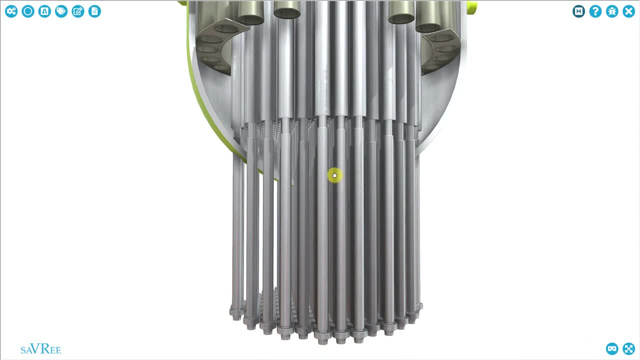 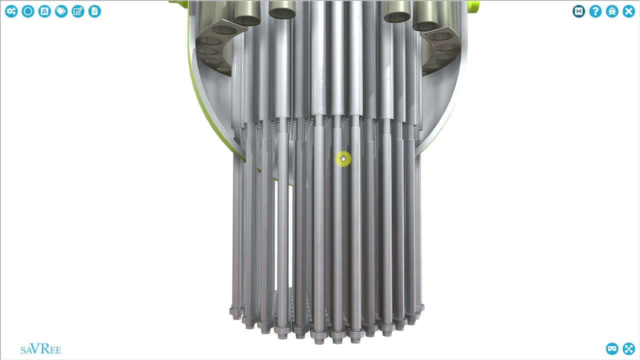 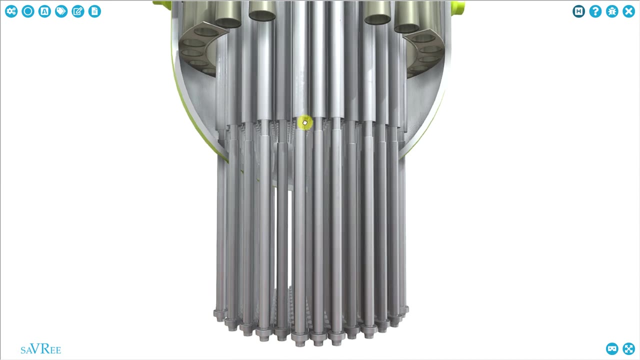 is that they're fed into the BWR from the bottom. whereas almost all other reactor designs feed the control rods in from the top and they'll fall due to gravity, The ones on this design are actually fed into the BWR using a hydraulic circuit. 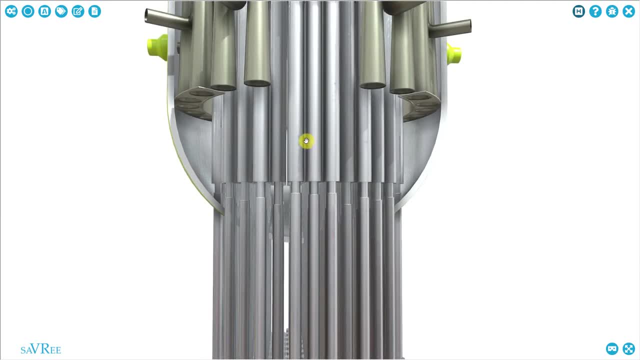 and you can use an accumulator, which is essentially a pressure vessel, as a way, in an emergency, to push the control rods in even if you don't have any electrical power, for example, when you have a blackout. Safety, as always, is a very big factor. 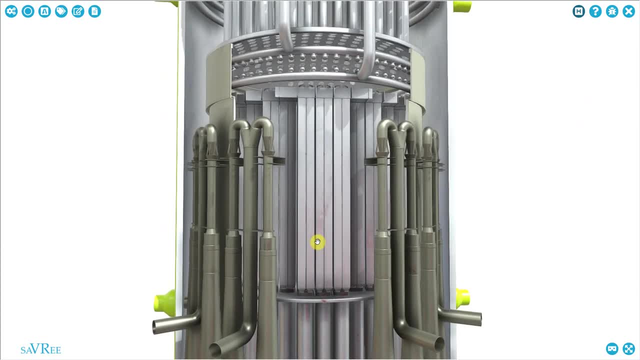 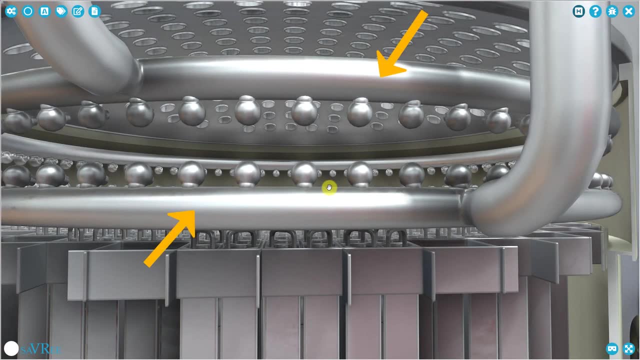 in a nuclear power plant, as it should be. So we've heated up our water. We come past these two sparge pipes here. These are for emergency cooling. We'll ignore those for the time being, Once we've passed through the fuel assemblies. 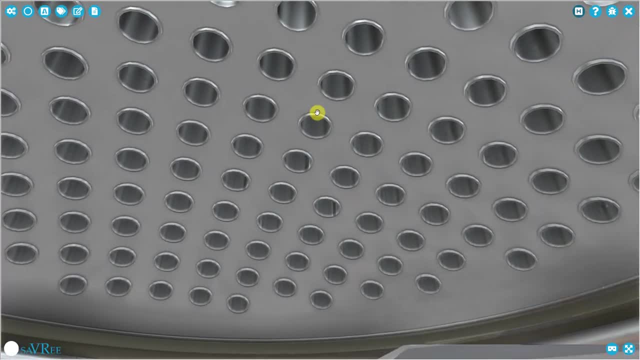 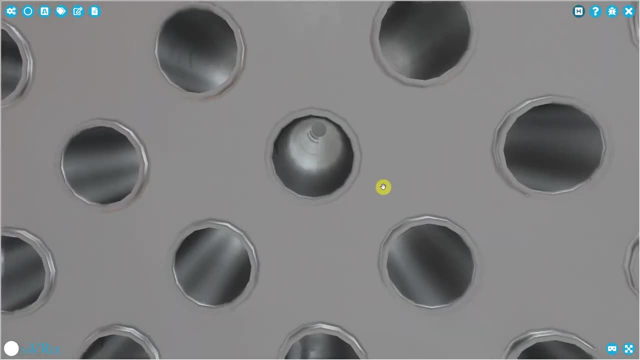 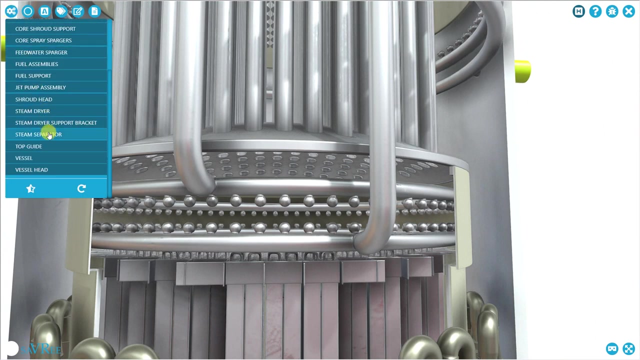 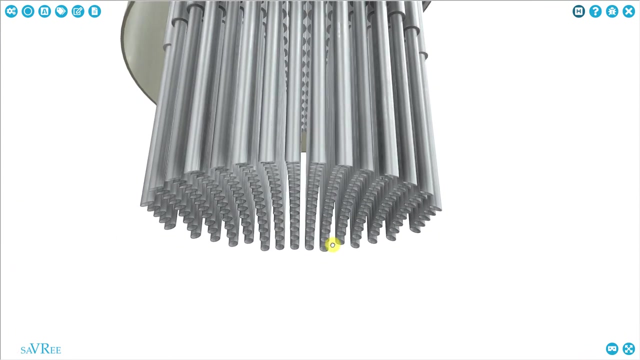 we get to the top of the shroud and the steam that's being produced is going to flow out of these tubes here, And these tubes help us to separate the water from the steam. What I've actually done now is configured the model to show you how these connect to the top of the shroud dome. 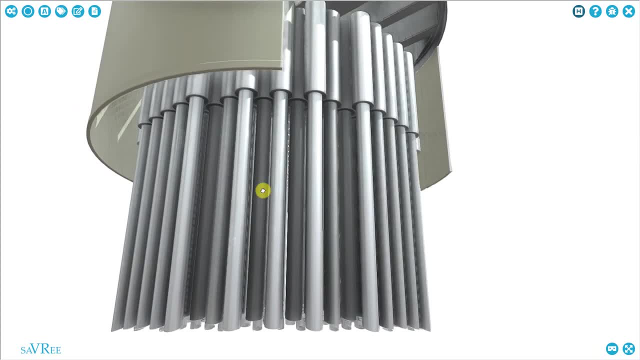 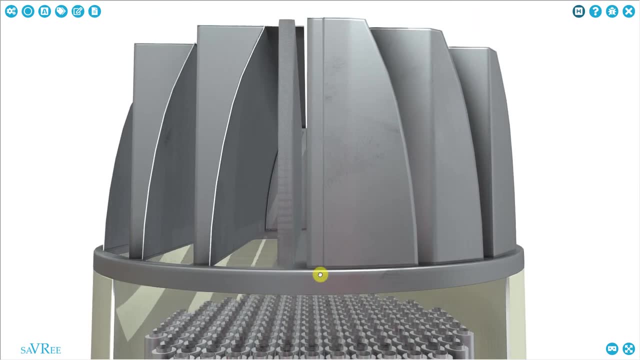 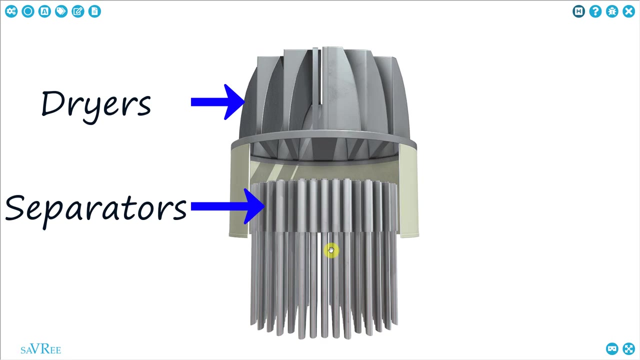 And you can see that the steam would rise up through the stand pipes, through our steam separators- so these sections are here- and then through our steam dryers up here. So why do we have all this? We have this because the steam is quite wet. 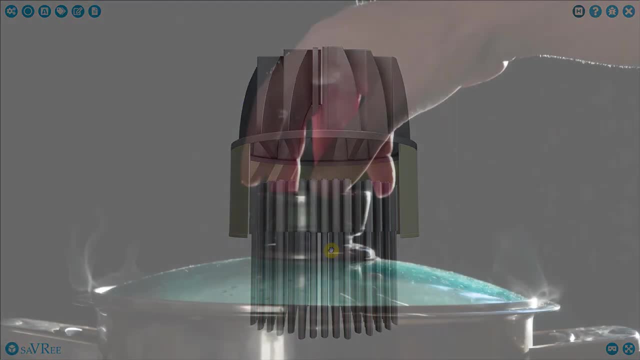 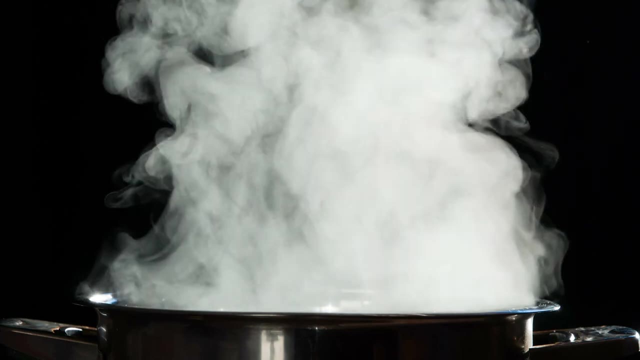 When you think of steam, you might think of it as having a white, fluffy, cloud-like appearance. You can't see steam in reality. Steam is a gas. Steam is a gas, And what you're seeing when you see the steam come out of the kettle. 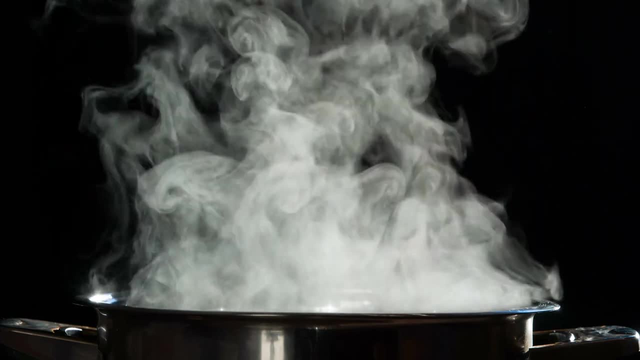 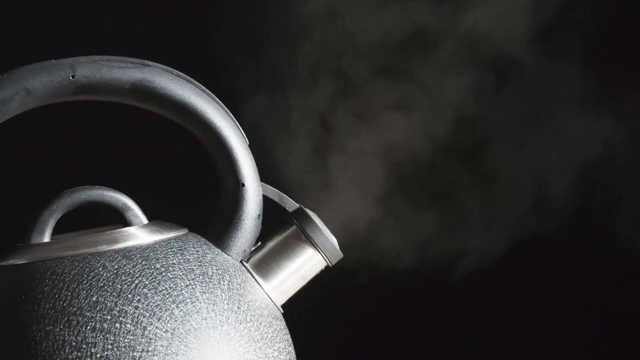 is actually moisture droplets, that's to say liquid water suspended in the steam. If you remove these water droplets, then you will not see the steam. If you remove all the water droplets, then the steam is considered dry. If you have many suspended water droplets, 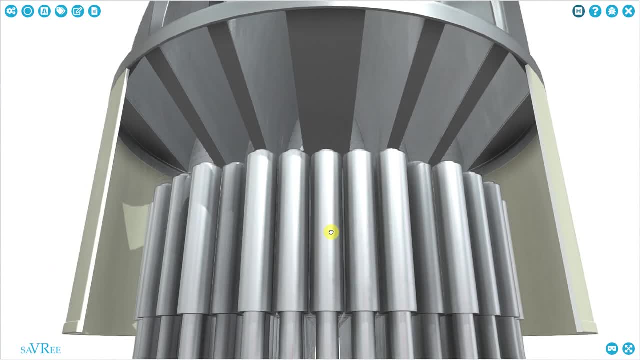 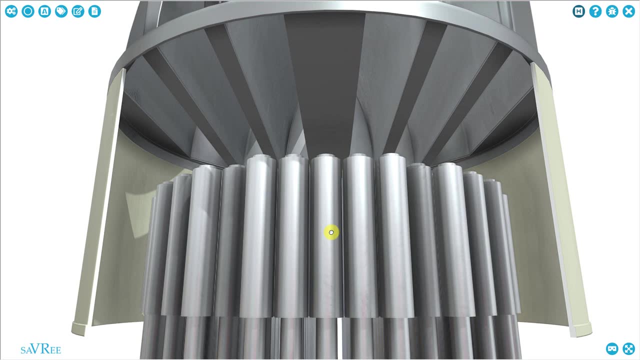 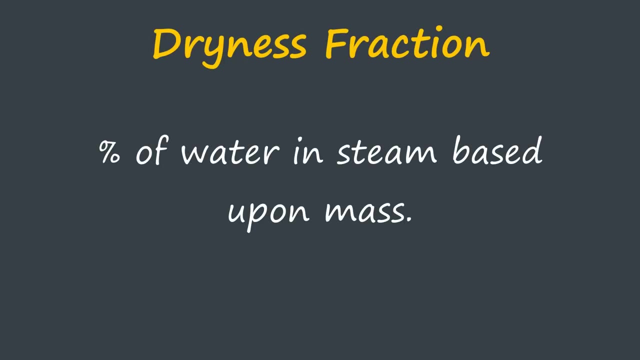 then the steam is considered wet. We pass the steam up through the stand pipes and the steam separators to separate out this moisture that's suspended in the steam. When we do that, the dryness fraction of the steam increases because it's drier than it was before. 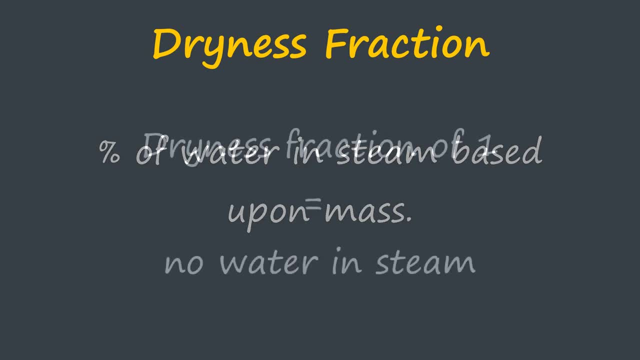 A dryness fraction of one indicates that the steam is dry. Less than that indicates that the steam is wet. The way we separate out the water from the steam is by letting it flow through a series of veins that are within these pipes, and these veins, in part, swirl onto the steam. 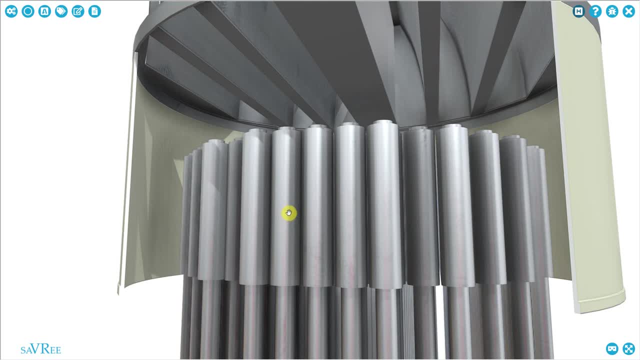 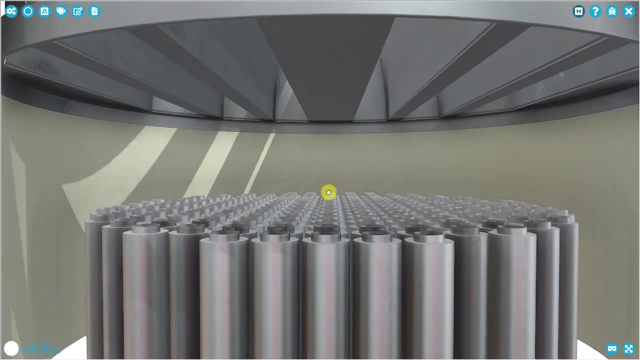 and the heavier liquid then condenses and begins to form on the outer periphery of these pipes. We can then drain off the liquid but allow the gas, the steam, to continue flowing through, Even when the steam flows out of all of these stand pipes. 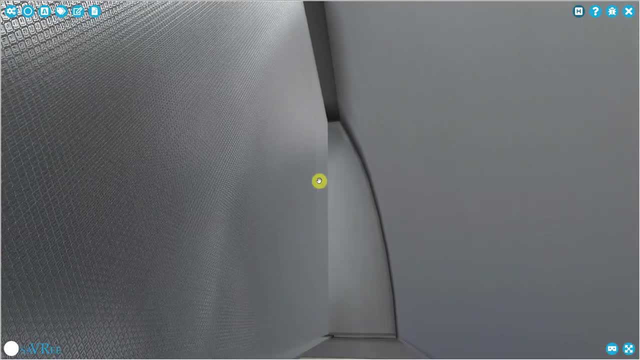 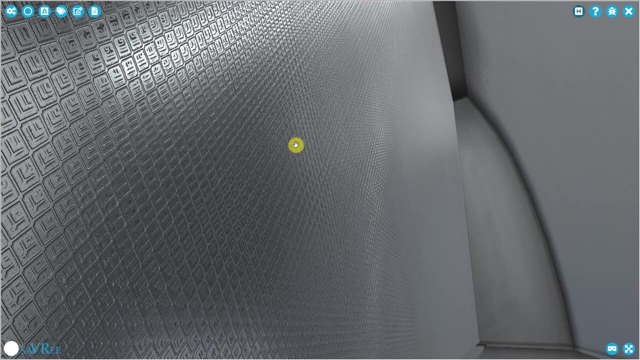 it still then has to flow through our steam dryers, and our steam dryers represent a tortuous flow path. You can see they've got this grid-like pattern here. This represents quite a hard flow path for the water molecules to flow through. Gas is much lighter and less dense, so it flows through far more easily. So the steam, which is gas, will flow through and most almost all of the water molecules within the steam will not. So we're separating out more moisture again from the steam.